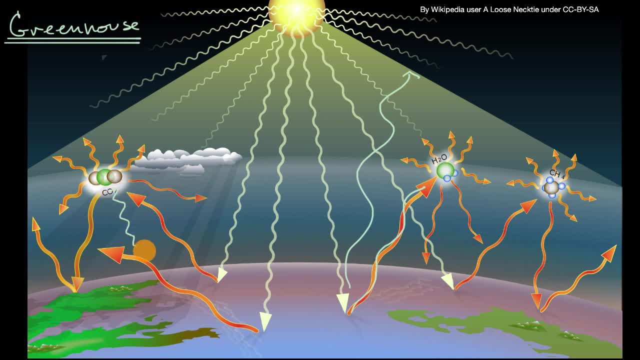 by these molecules, by these gases, and then they will emit some of that back to earth, And so that's why it's called a greenhouse effect, because of all of that energy that might have been sent out to space if you didn't have an atmosphere. not all of it is. 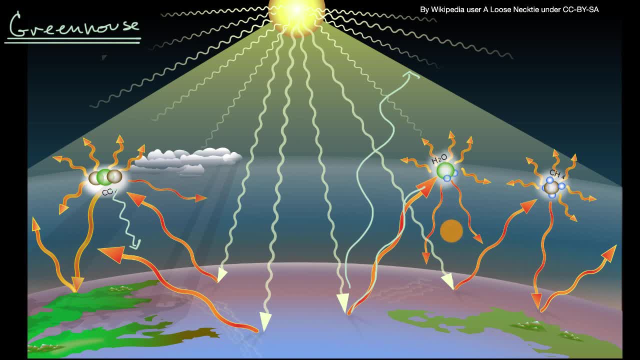 Some of it is reabsorbed by the atmosphere, which then sends it back down to the surface, and that process can go on and on and on. You can imagine that it's trapping some of the energy Now: the greenhouse effect and greenhouse gases. 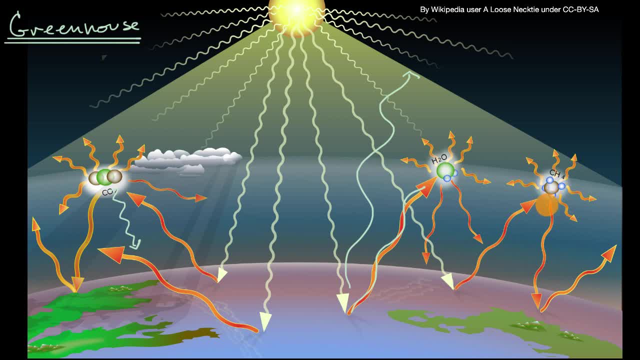 the ones that I just listed. they're oftentimes associated with manmade climate change and global warming, And they are for good reason, but it's important to realize that we actually need some base level greenhouse effect just for earth to be habitable in the way that it is. 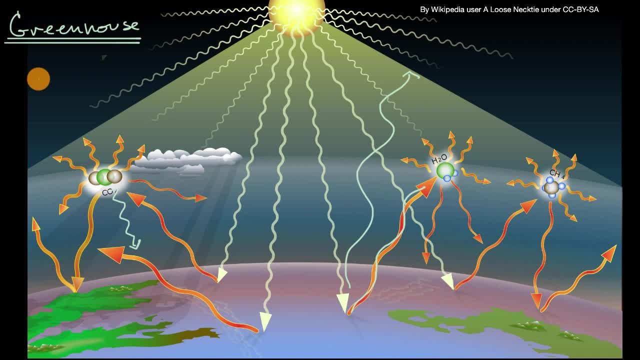 Without greenhouse gases, earth's surface would be about negative 18 degrees Celsius, which is the same as zero degrees Fahrenheit, which I think most of y'all would recognize is very, very, very cold relative to what the actual averages are, which are 15 degrees Celsius or 59 degrees Fahrenheit. 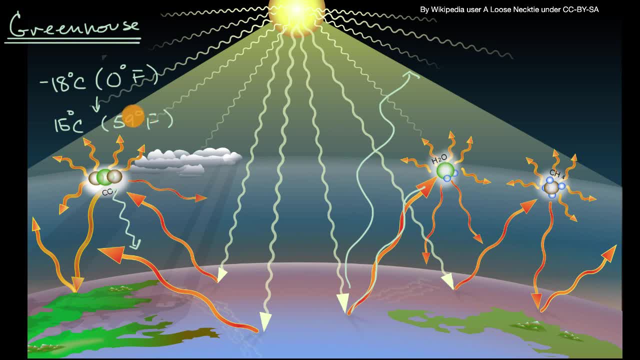 And of course these are average temperatures. but 59 is a nice, refreshing brisk day, not a frigid day like zero degrees Fahrenheit. And of course these are averages. It fluctuates around this depending on time of year and where you are. 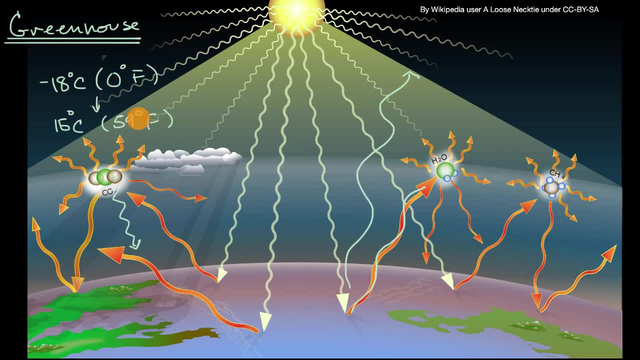 But this just makes it clear that we do need these greenhouse gases to keep the earth reasonably warm. Now the problem is is if the concentration of these greenhouse gases go out of equilibrium, become unusually high, and it does look like that is indeed happening. 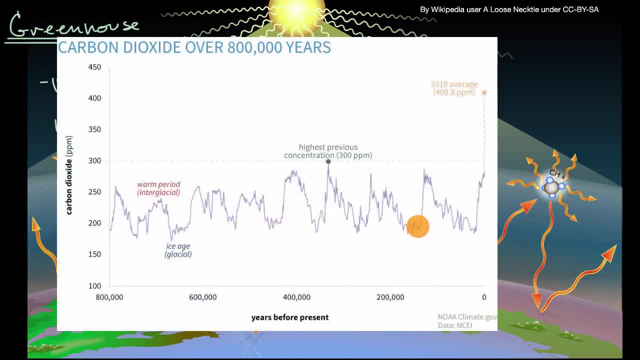 This right over here is a chart, and the way that we're able to figure that out is by taking ice samples and rock samples and looking into our past through the geologic record of how much carbon dioxide there has been over the last 800,000 years. 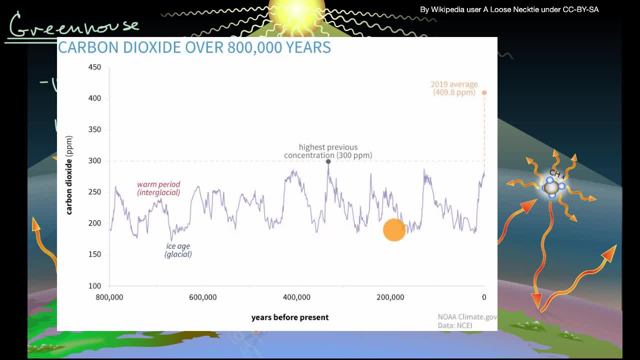 And 800,000 years is a very long time period. Modern human beings have only been around for two or 300,000 years, And what you can see is the concentration of carbon dioxide has roughly fluctuated between about 200 parts per million. 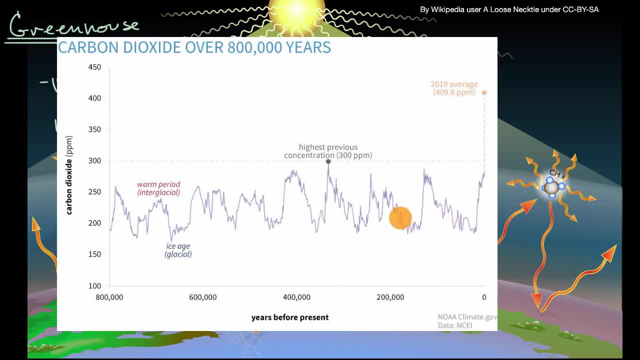 and about 300 parts per million at least over the duration of this chart. But in recent times we've gone well beyond that, We've almost gone, we've almost doubled that average right over here, And this is actually the highest levels we've seen. 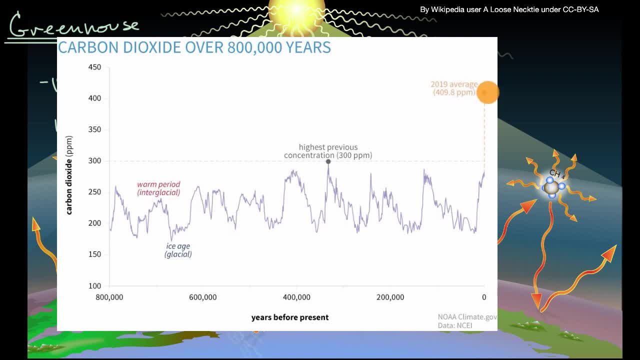 in three million years. Now it's important to realize that carbon dioxide makes up a small percentage of our atmosphere. In fact, all of these greenhouse gases make up a small percentage. 78% of the troposphere is nitrogen, 21% is oxygen. 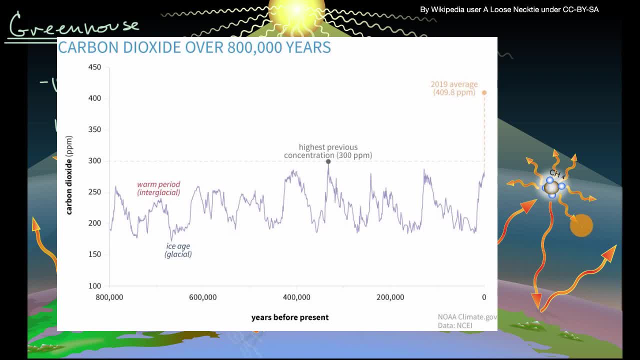 The last 1% is things like argon, water vapor, carbon dioxide, methane. So even this small amount, when the concentration increases dramatically, can have a huge effect. Now you might say, hey, we were at these levels three million years ago roughly. 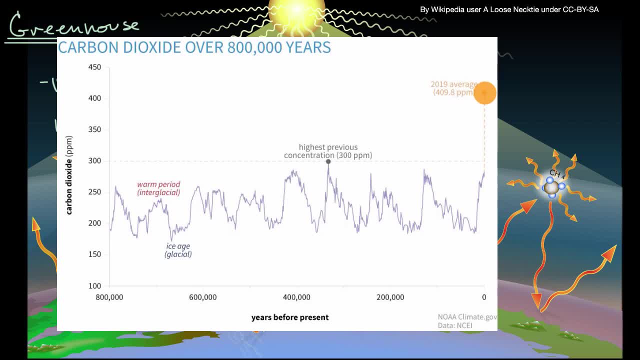 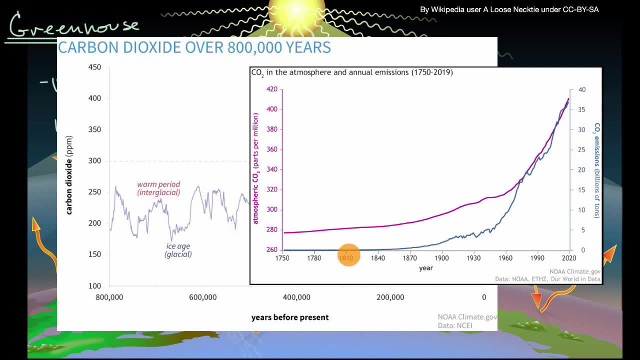 Maybe this is just some type of cycle that we're seeing on Earth, And to recognize that this is indeed manmade, we just have to look at a chart like this. This tells us two things. This tells us annual emissions in this blue line. 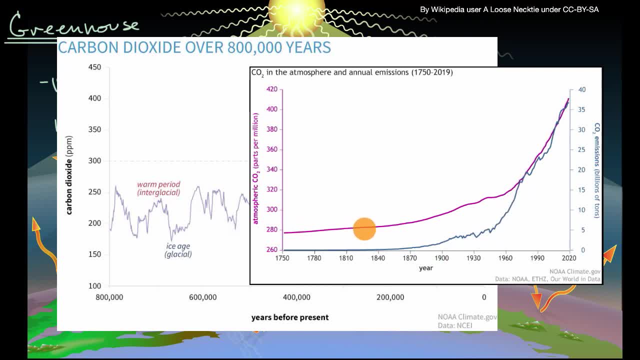 this blue curve and then the total emission or the total concentration in the atmosphere, Because one of the thing about you know, about one of the things about a greenhouse gas like carbon dioxide: when it's emitted it doesn't just disappear. 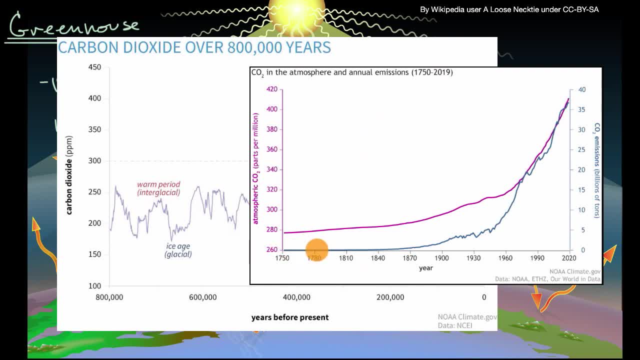 And we can see if we go to the pre-industrial revolution or the early stages of the industrial revolution. CO2 emissions were pretty low, pretty close to zero, at least on this scale. right over here There might've been some basic CO2 emissions. 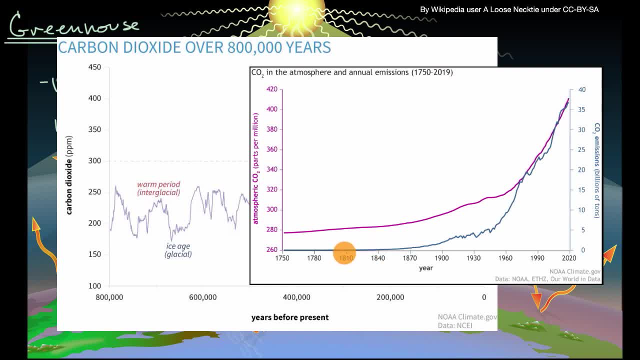 People had fires and stoves and things like that. But then as the industrial revolution came into play and we started using fossil fuels more and more to fuel transportation and factories and other things, our emissions have gone up dramatically And this coincides with the total concentration. 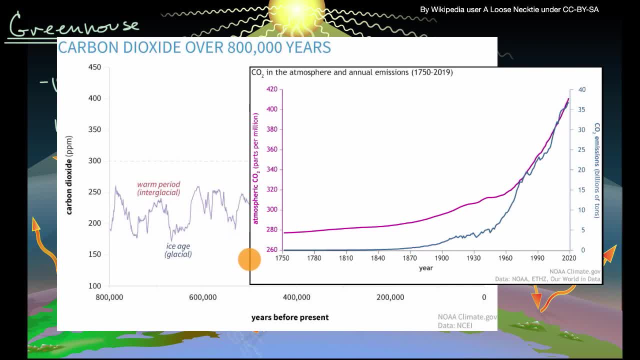 going well above that 800,000 year average. So it's important to keep in mind. the greenhouse effect is needed to some degree, But the problem is is when the concentration of greenhouse gases like carbon dioxide go well beyond their historic averages. 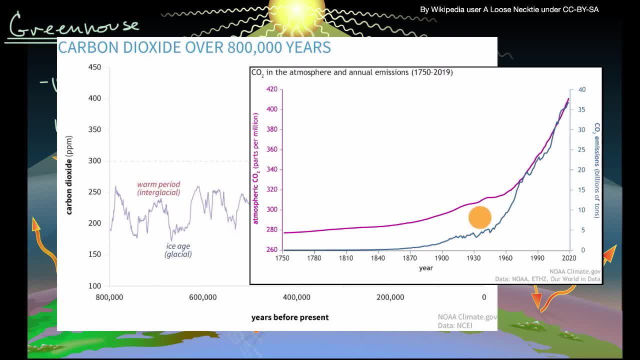 which can, over time, warm the earth, And even a few degrees centigrade of warming the earth can have huge consequences on our environment and on our weather. I brought one last idea just for kicks, because, even though it's called the greenhouse effect,